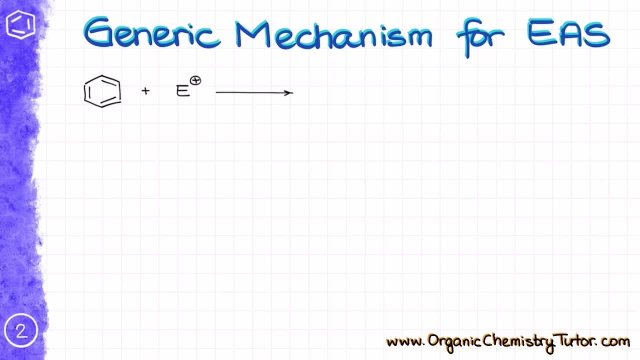 need to know about our electrophile is that it is a strong one, and the reason why we need a strong electrophile is because aromatic compounds are very stable. So if we want to attack the pi system and break that aromaticity, we'd need something very strong to do that, And once that 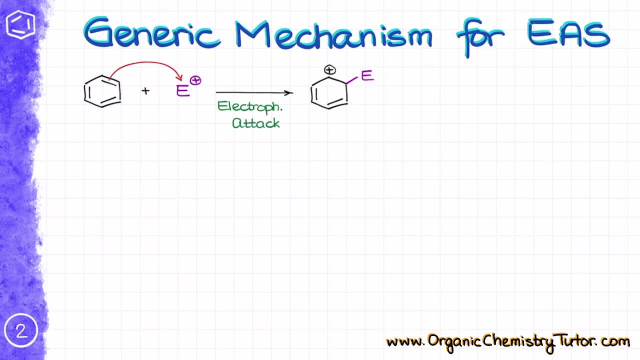 happens, we're going to end up with a carbocation. This carbocation is resonance stabilized, so we can draw three resonance contributors for it. There will be a lot of resonance drawing in this topic, so if you are not feeling very comfortable with the resonance or need a refresher, 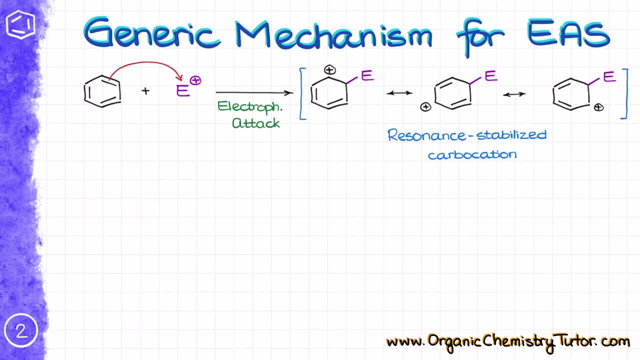 make sure you review it now. We're going to be using resonance as one of our main tools of investigation here, so it's crucial you are capable of using that and be very comfortable with it. Alright, so now back to my resonance. stabilized carbocation- We occasionally call this. 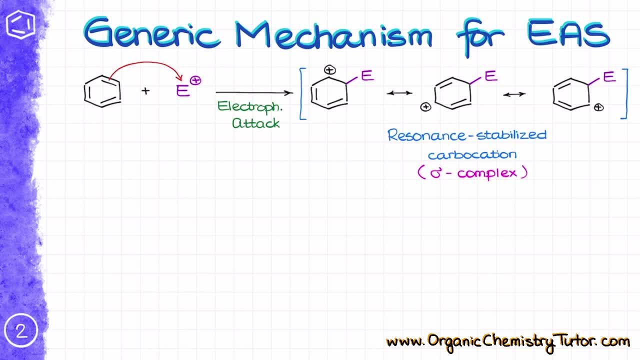 intermediate, a sigma complex. The sigma complex is an outdated term, but it was very popular in the middle of the last century and you can still see it in some textbooks up to this date. So what are we going to do? Well, once we have our carbocation, we have a bit of a problem on our 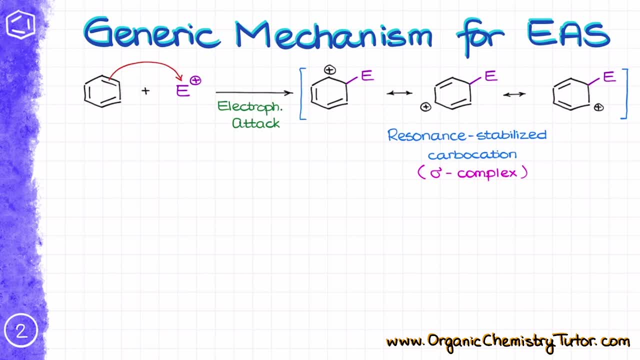 hands. You see, to make this carbocation, we had to break the aromatic ring and thus we lost the stability that comes with it. And, as I've mentioned in my previous tutorial on aromaticity, molecules will do whatever it takes to regain aromaticity or to maintain it. This intermediate is no exception. 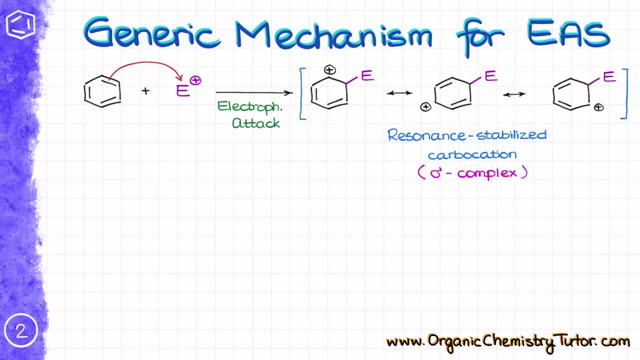 but what are we going to do to make our molecule aromatic again? Well, we can lose the proton from the position where we've attached our electrophile. this proton, And this proton is incredibly acidic. It is a proton on a carbocation, and we know that carbocations are wickedly acidic. 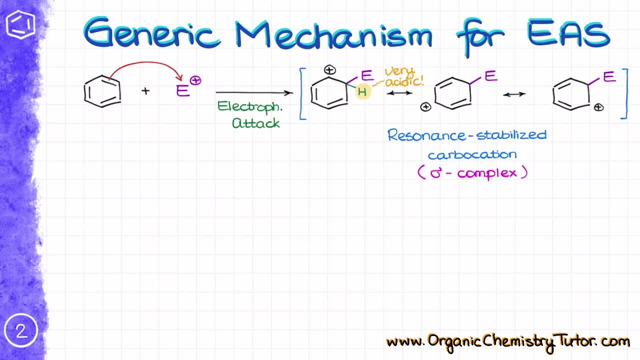 Also, the removal of this proton restores aromaticity, so it will be a very thermodynamically favorable process if we were to get rid of it. So some sort of a conjugate base again. the nature of that base is irrelevant for the moment. 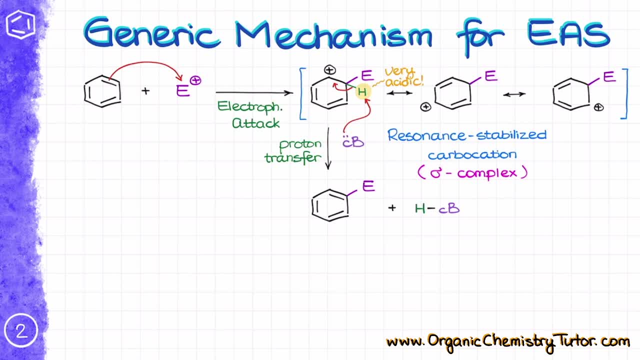 That base will come and pull off the proton And due to how acidic the proton is, we don't really need anything very basic. Essentially, anything with an electron pair will do. Even another aromatic ring by itself can do that. And here is an important thing I want to point out before we. 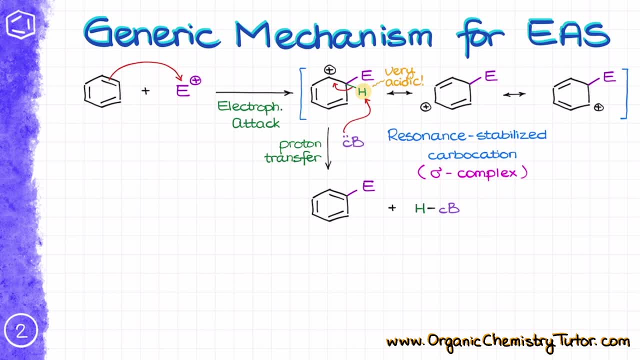 move any further. While this reaction might look like some sort of addition because we just added an electrophile to our molecule, it is not. If you pay close attention to what's been going on in the molecule, you'll see that the reaction is not so good. It's not so good. It's not so good. 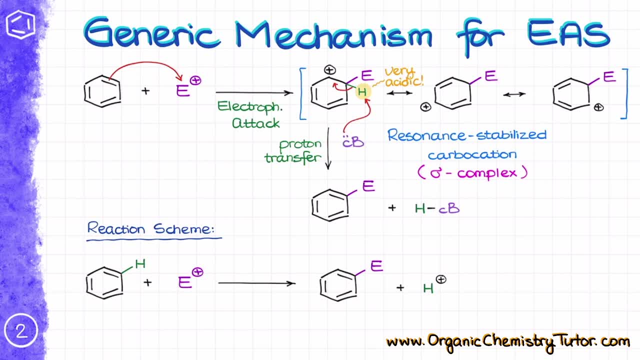 You can see that there was a hydrogen right over here on our molecule And that hydrogen in the course of the reaction we replace that hydrogen with our electrophile. So while we don't normally consider hydrogens as living groups in this reaction, it essentially plays a role of one. 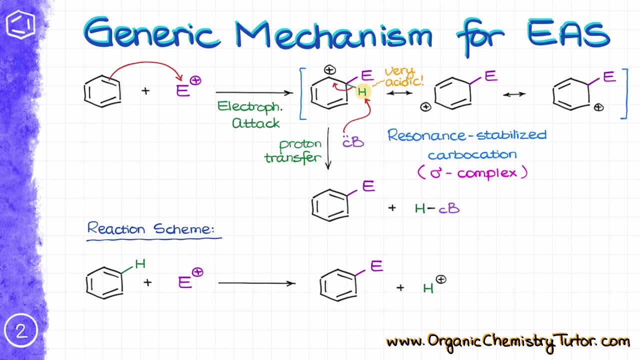 by being replaced with the electrophile. Therefore, it is a substitution reaction, although it may not look like one, especially if we are writing the reaction using the skeletal structures without showing the implicit hydrogen atoms. All right, now let's look at the actual electrophilic aromatic. 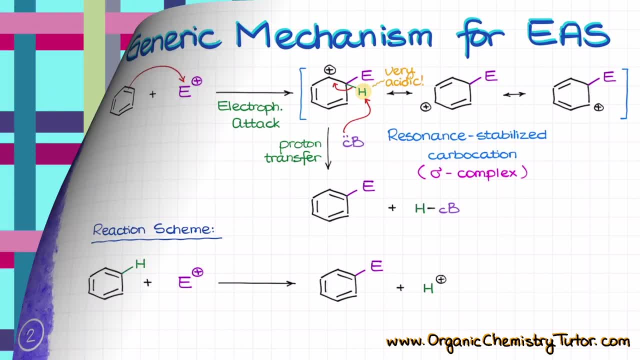 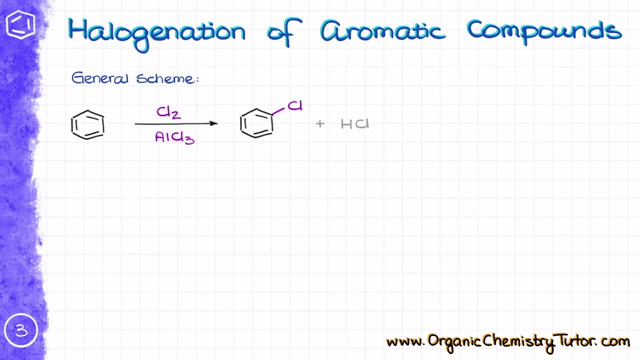 substitution reactions I've mentioned at the beginning of this video, And we'll start with the halogenation reaction. In the general scheme we see that we need a halogen. I'll be using chlorine here and another species, aluminum chloride. Aluminum chloride is the catalyst that we need to. 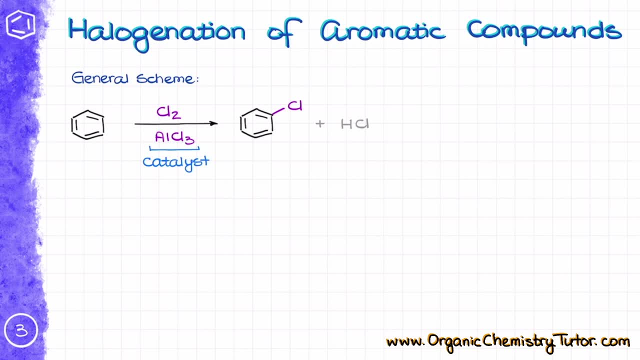 make a good electrophile And as a catalyst it's not going to be consumed in this reaction. So once we start working through the mechanism of this reaction, we'll have to make sure we regenerate that, And the first step in this reaction is going to be the formation of our 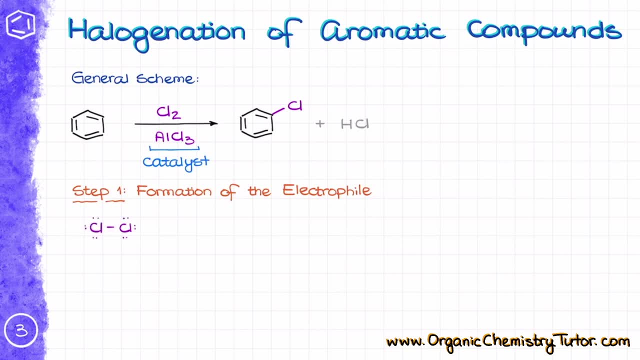 electrophile, And while chlorine is electrophilic, it is not electrophilic enough to tackle the aromatic ring and disrupt aromaticity. So this is where the aluminum chloride comes in. Many metal chlides are good Lewis acids, meaning they're good at accepting electrons. Aluminum chloride is an 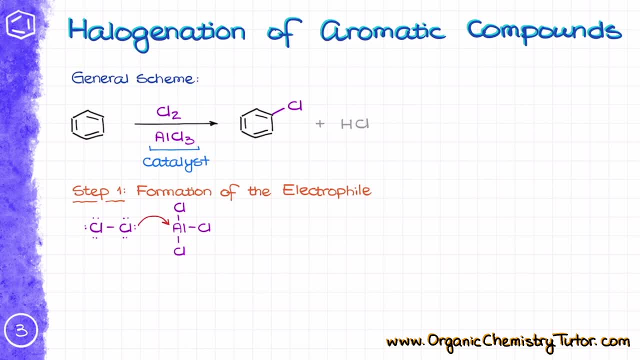 exceptional Lewis acid. So it will pull the chlorine towards itself to steal some of its electron density. This will yield a new complex between the chlorine molecule and aluminum. And because chlorine has to provide some of its electron density to make this bond the new bond, 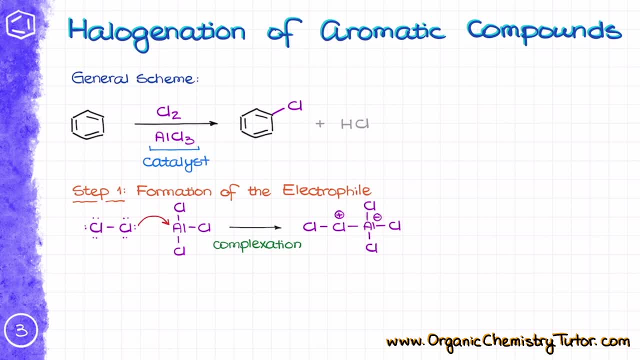 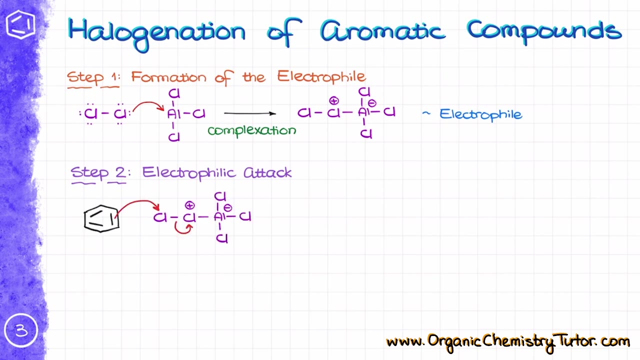 that we have between aluminum and chlorine over here. this makes chlorine very electrophilic because it is now electron depleted. Now this new complex is going to be our electrophile And in the next step we're going to be doing our electrophilic attack In this step, our newly made electrophile attacks. 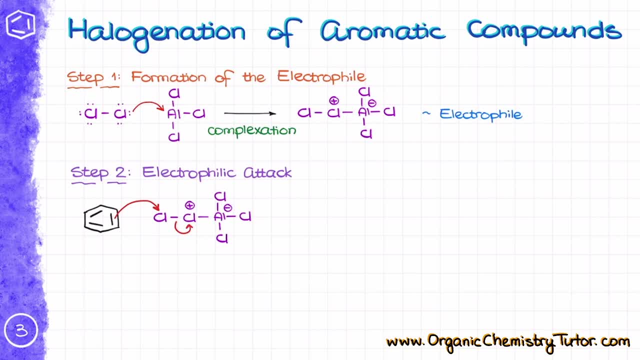 the aromatic ring. Notice that in this attack it's the chlorine atom on the edge of the molecule over here that's actually doing the attacking and not the one with the formal positive charge. So the attack goes from the aromatic ring on the edge- chlorine. 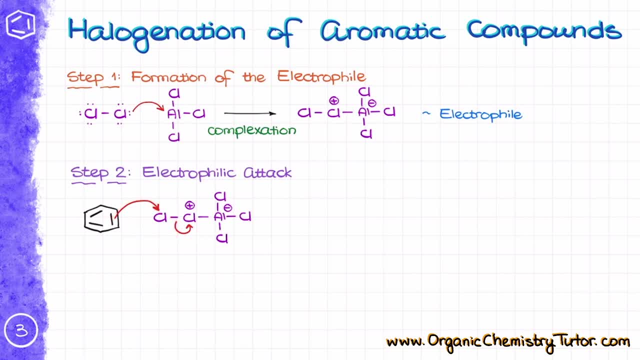 and that breaks the bond between our chlorines. This attack results in the formation of our resonance-stabilized carbocation intermediate, or the sigma complex, if you like that name better. And finally, we're going to restore the aromaticity by removing the proton from our 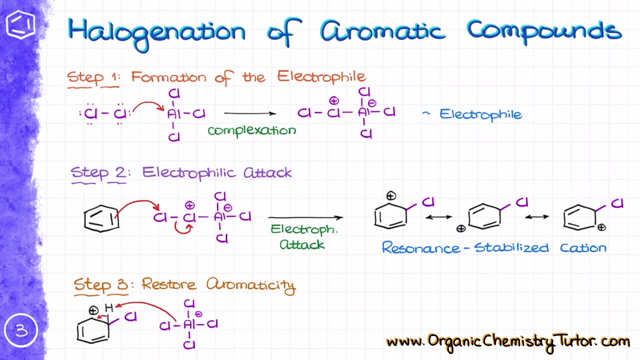 carbocationic intermediate, And as a conjugate base, we're going to use the leftover of our catalyst that now has an extra chlorine atom. That gives us the final product, chlorobenzene in this case, and the regenerated catalyst, along with the HCl, which is the core. 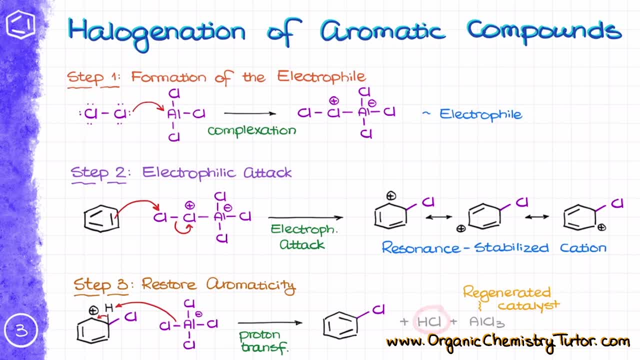 product. We don't really care about this part and, as a matter of fact, you're probably not even going to mention that when you are writing the mechanism And likewise, the catalyst will remember that the catalyst still exists and will regenerate that, but we are probably not going to be showing that. 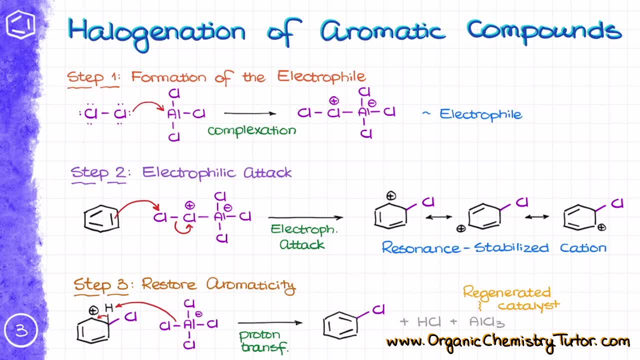 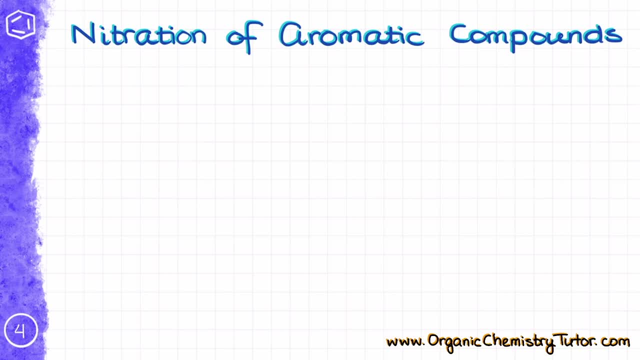 in the final mechanism for the test purposes or anything like that. So the next reaction in this series is going to be the nitration of aromatic compounds. In the general scheme, we can see that we have the main reagent, which is going to be our nitric acid, over here, and we also have the 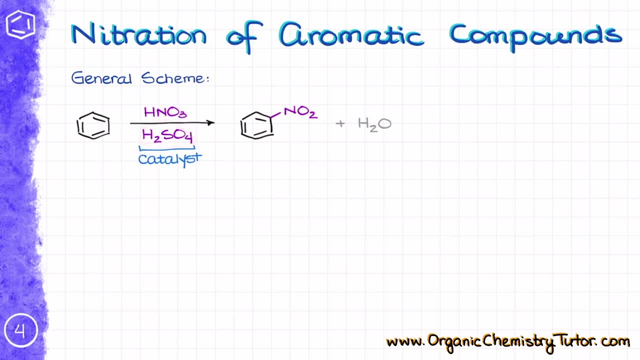 sulfuric acid over here, which is a catalyst, And, like in the previous case, the nitric acid is not electrophilic enough by itself and it cannot tackle the aromatic ring as is, so it needs a little help to become more electrophilic. And as sulfuric acid is a strong, strong, strong, strong, 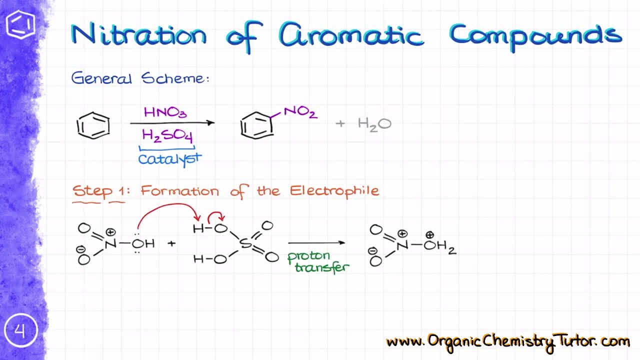 acid than the nitric acid. the reaction starts by proton transfer from sulfuric acid to the oxygen of nitric acid. This forms a rather unstable protonated nitric acid which quickly undergoes the leaving group dissociation, giving us the nitronium ion which is going to be our electrophile. 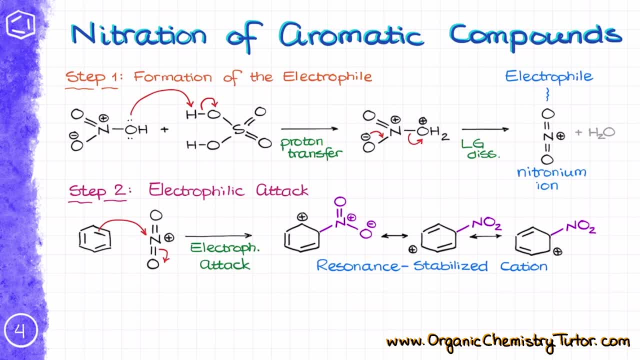 And as the nitronium ion is a strong electrophile, it will have no problems attacking the aromatic ring, making a resin and stabilized carbocation, just like we've seen in the previous scheme. I am not going to show the full Lewis structure here for the nitro group for the sake of space. 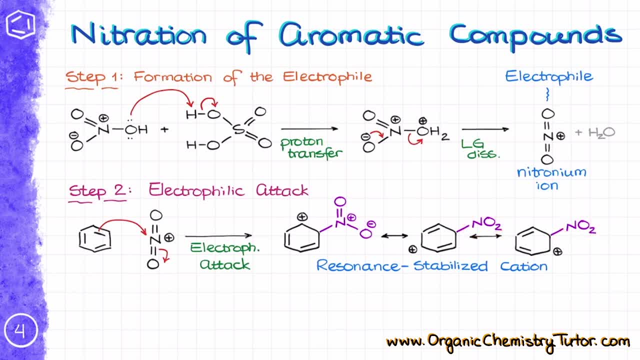 so I'll just leave it as NO2 here and here, but I encourage you to draw that on the exam in its full glory, as many instructors will really appreciate the fact that you actually know how the nitro group looks like, Jokes aside, but you have no idea how common this error is. 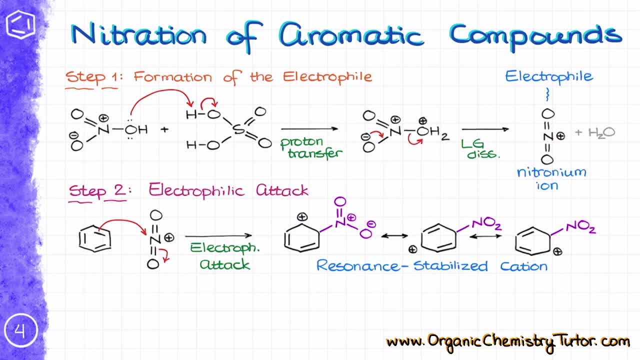 For whatever reason, students just don't remember the structure of the nitro group. It's me have no idea why. All right, I'll stop complaining here and let's get started. Let's move to the next step. So, once we have our carbocation intermediate, the last step. 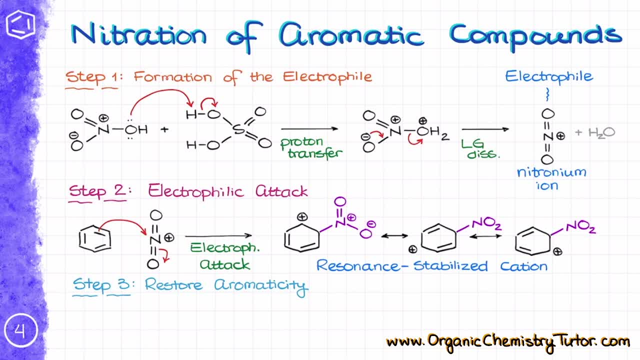 on this reaction is the aromaticity restoration via the proton transfer, like in the previous case again, And here we are going to be using the conjugate base left over from our sulfuric acid which is going to be regenerating our catalyst H2SO4 over here and giving us the 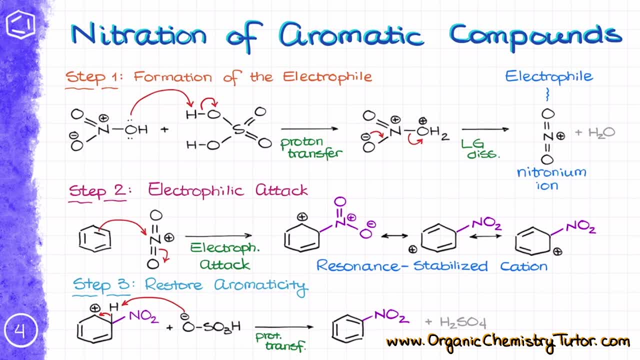 final product, which is nitrobenzene in this case. Nitration, by the way, is a very important component of this reaction and we never want to perform it on a sensitive and a very complicated molecule. The nitric and sulfuric acids together can pretty much eat throughout just about. 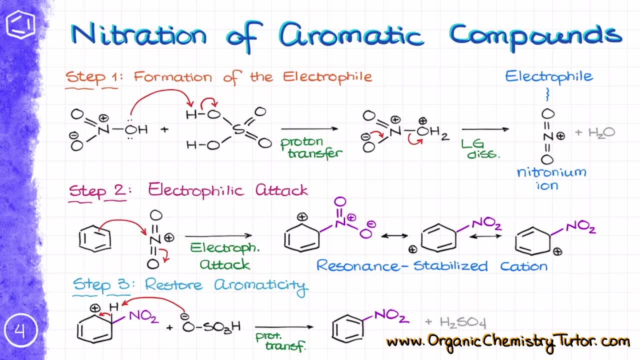 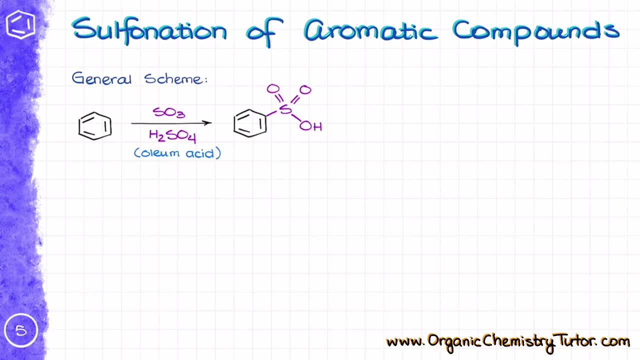 anything. So many functional groups may be destroyed in this reaction if we are not careful. So next we have the sulfonation reaction, And in this reaction we are going to treat our aromatic molecule with a fuming sulfuric acid, which is the solution of SO3 in concentrated sulfuric acid. 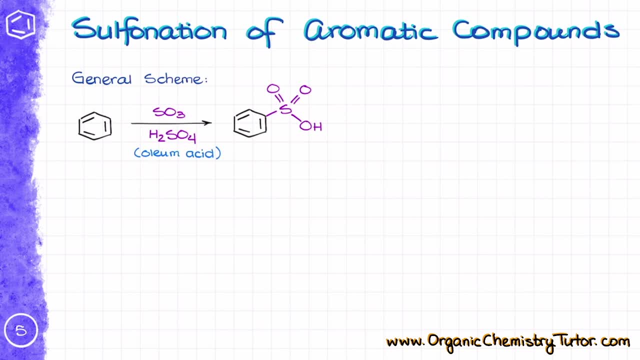 This mixture is a thick, viscous yellow-brown liquid and, because of its consistency and because of how it looks like, it is sometimes called the oleum acid. The reaction results in a sulfonic acid and, interestingly, there are no co-products in this reaction, so don't accidentally draw water. 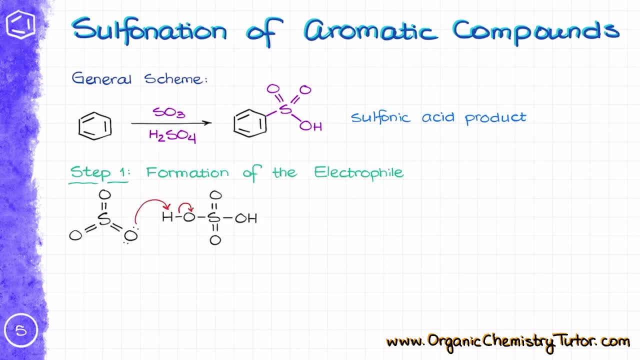 or anything like that as a co-product, because there are none. As always, we're going to start our mechanism with the electrophile formation, and in this case it's going to be the protonation of the SO3. This gives us the electrophile that will then attack the aromatic ring Again here, the SO3, by. 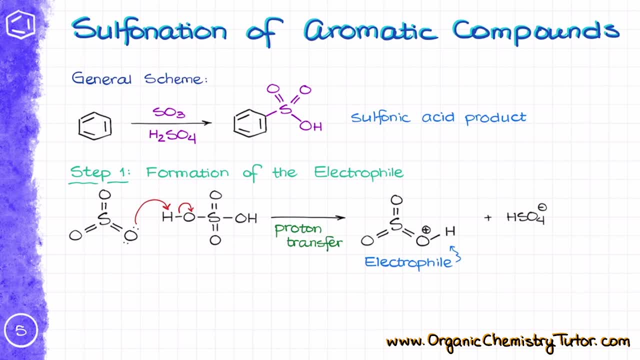 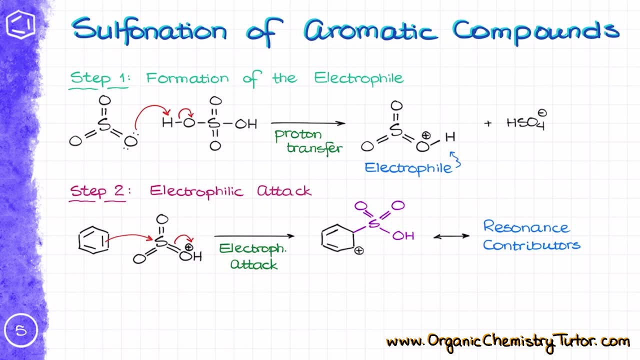 itself is just not strong enough to attack the aromatic ring, so we need to take it over the edge by protonating it. The electrophilic attack in this reaction gives us our typical carbocation intermediate, As this is already the third time we are seeing the same style intermediate in this. 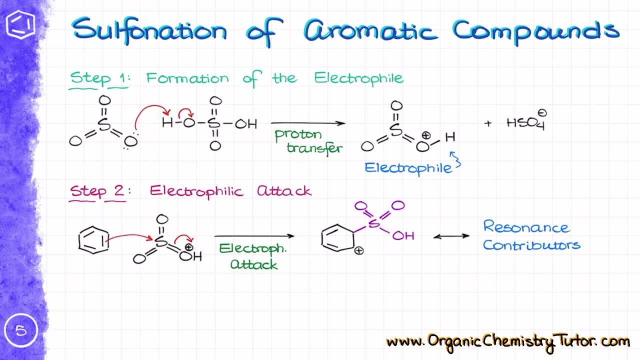 tutorial. I am not going to show all the resonance structures, so try drawing them out and see if you can do it on your own. You can use the other two examples that we have already seen as the template for the resonance structures. So, finally, we are going to restore our aromaticity by removing the proton from our carbocation. 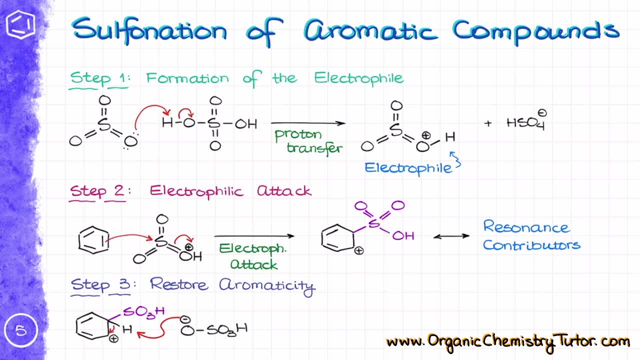 In this reaction, we're again going to be using the sulfuric acid conjugate base for these purposes, And that yields us our final product, the sulfonic acid. And here is something really interesting about this reaction: it is actually reversible, unlike the previous. 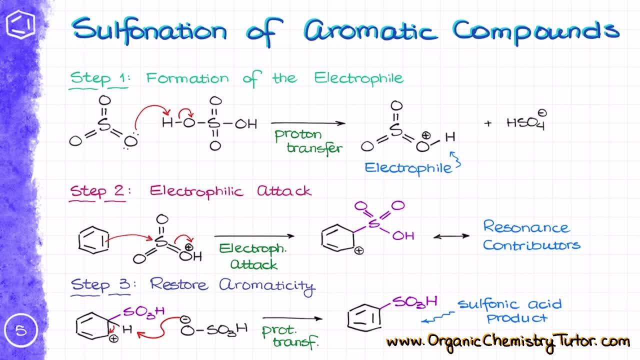 two. This means that we can also remove the sulfonic acid group if we do this reaction in a dilute sulfuric acid solution. As a challenge, I encourage you to come up with a mechanism of this reaction on your own, using all the same steps, but do them in the reverse order. And why is it? 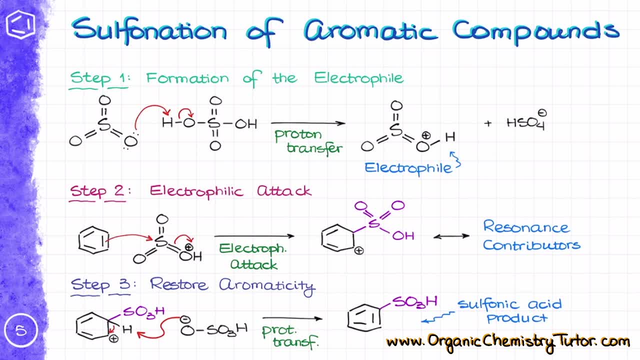 important to know. Well, later in your course you'll start talking more about the multi-step synthesis, and this reaction becomes a useful trick which you can use to temporarily block anything. do some other chemistry and then remove the temporary block when you no longer. 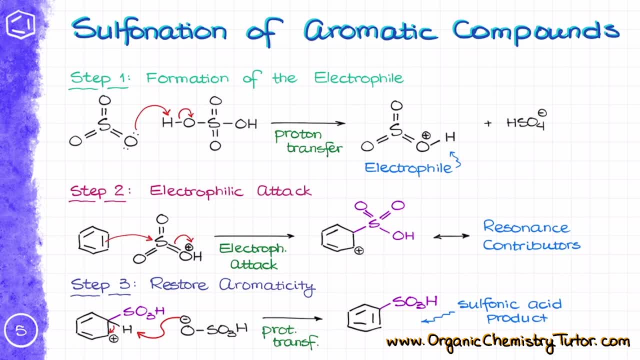 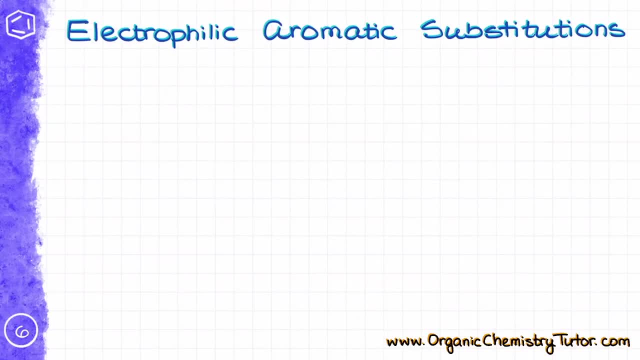 need it. So it sort of acts as a protecting group for the position in the aromatic ring. so nothing else going to go there. Let's do a quick review of what we've just learned. If we treat an aromatic compound with a halogen, either a chlorine or a bromine, in the presence of the Lewis acid catalyst, 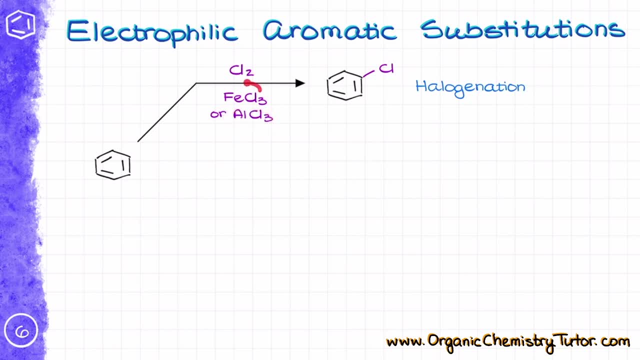 such as the aluminum chloride, which we have already seen, or iron chloride, we are going to end up with the halogen neutral, So we're going to replace one of the hydrogen on the aromatic ring with the chlorine or bromine. correspondingly, If we treat an aromatic compound with a nitrating mixture, which is 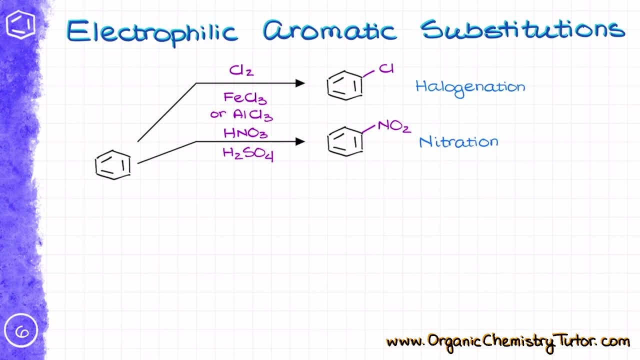 the mixture of concentrated nitric and sulfuric acids, we're going to get a nitrated aromatic compound and we call this reaction the nitration. The treatment of aromatic compounds with the fuming sulfuric acid results in the sulfonation reaction and I'm going to remind you here: 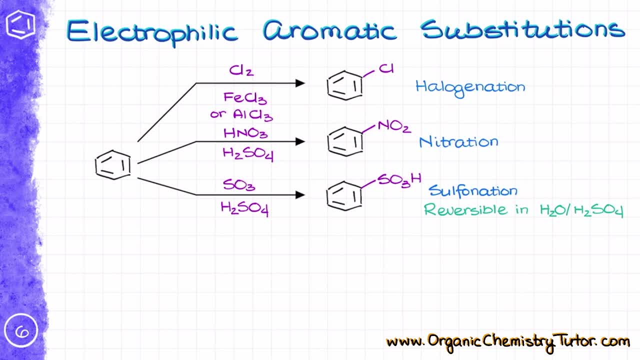 that that is a reversible reaction, so we can take the sulfuric acid group off from our molecule when we no longer need it. Finally, we have the Friedel-Crafts alkylation and acylation reactions. I haven't talked about those two reactions in this video, for a very good reason: They are much more complicated.